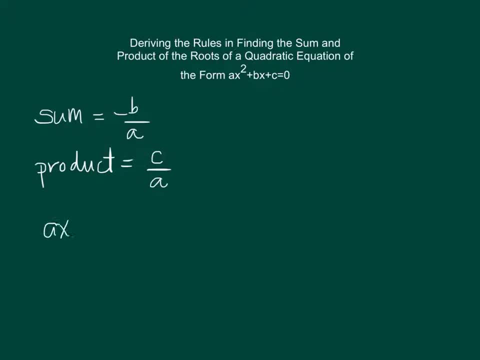 So let's start with the quadratic equation itself. So ax squared plus bx plus c is equal to 0.. Now note that this equation can be transformed into: x squared plus b over ax, plus c over a is equal to 0 if we multiply the equation by 1 over a on both sides. 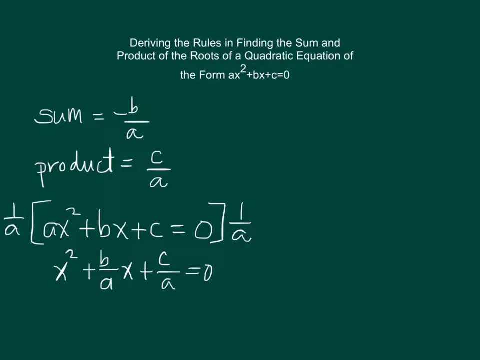 Now, as we solve for the value of x, we could expect that this equation will be transformed into its factored form. that will help us determine the values of the roots. Now let's say, for example, that if we continue to solve for those roots and ended up with the following roots, namely r1 and r2.. 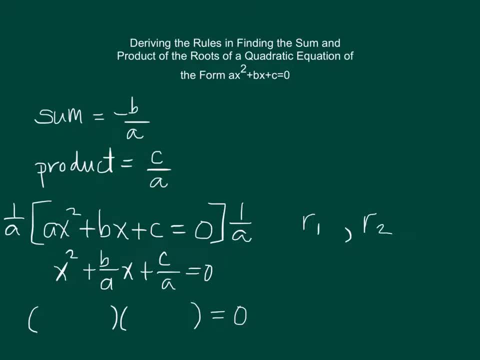 So the factored form of x squared plus b over ax, plus c over a, is equal to 0, should take the form of x minus r1 and x minus r2.. Now this is very critical in understanding how the rules were derived, because we have to take note that x minus r1 times x minus r2 is just the factored form of x squared plus b over ax, plus c over a, is equal to 0.. 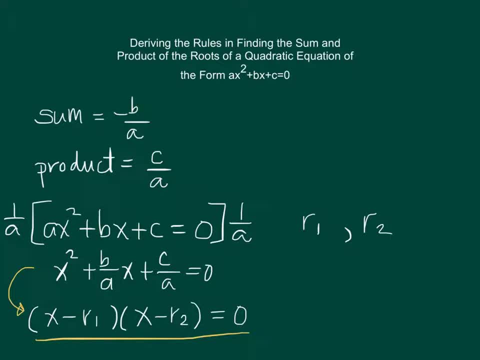 Since it is the factored form, they must be equivalent. Okay, so take note they are equivalent And that, if I simplify, x minus r1 times x minus r2 is equal to 0, it should have the form: x squared plus b over ax, plus c over a, is equal to 0.. 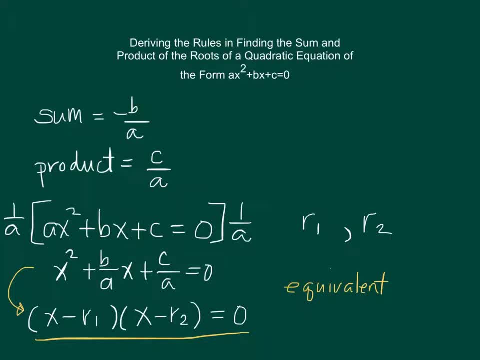 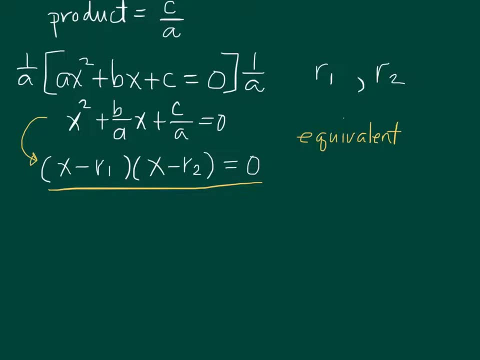 Okay, that's very important. So, as we continue, now let us expand x minus r1 times x minus r2.. So if I will expand this, this will become: x squared Minus r2x minus r1x, plus r1 times r2 is equal to 0.. 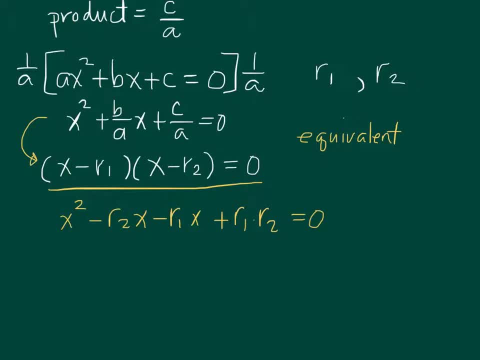 Now we could have many different ways of expanding it And we will still be having the same expanded form. Okay, so this expanded form can be transformed into x squared minus r2 plus r1.. So what we want is if we have the square of 1x plus r1 times x plus r2, which is equal to 1x. 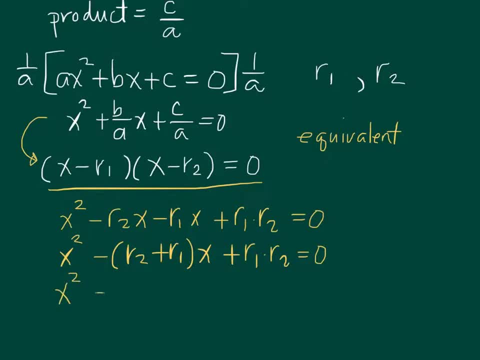 Therefore we have the figure of the平en. So the formula is: we have dla the f sheet 1st plus delta sheet 3, 1th plus delta sheet 2, th. we have b over c squared plus b over a delta sheet, which is equal to 1x plus the. 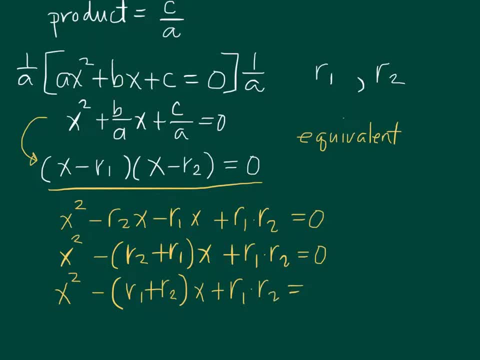 f side им, We have the square of 2x plus b over a delta sheet is equal to 3 x plus delta sheet. 2 switch to delta and the two sensing values could be d to the 3 complete elements in this equation. 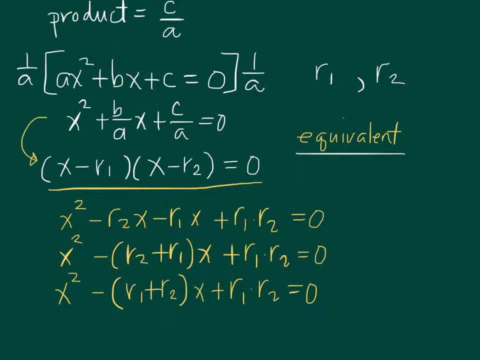 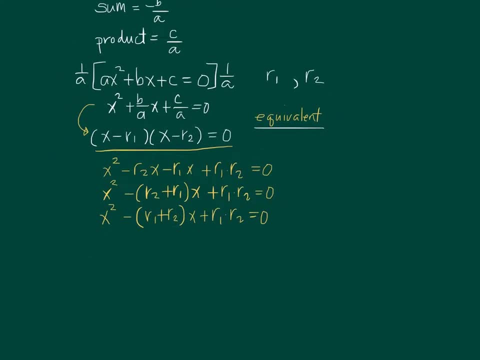 We have 2ения, b, b, c, dash, M, X again. so this sytem here And now the 15. touch which I wanted to write here. See if I will have. now the other equations be written just under the expanded form of x minus r1 and x minus r2,. 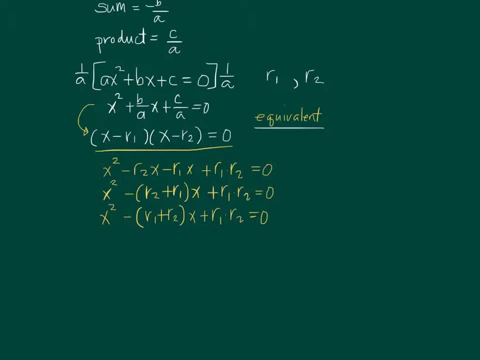 you will clearly see the relationships of the roots to that of the coefficients a, b and c. Okay, so we have. so let's bring this down here. So we have: x squared plus b over a. x plus c over a is equal to 0.. 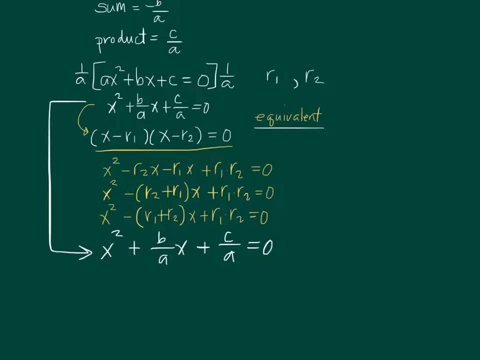 Since they are equivalent, then we could correspond the terms of the expanded form of x minus r1 times x minus r2, equal to 0, to that of x squared plus b over a. x plus c over a is equal to 0.. In short, b over a. 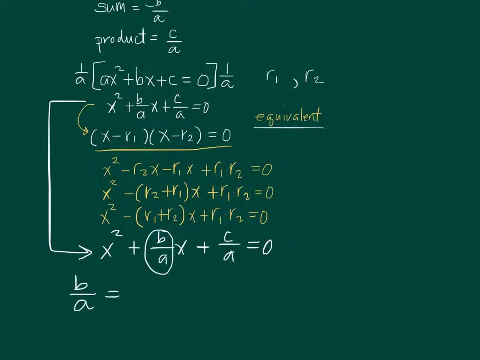 b over a should be equal. so this is, the b over a should be equal to negative r1 plus r2.. And that c over a must be equal to r1 times r2.. And if you see it now, this is taking us to the two formulas that help us to find the sum and the product of the roots of the quadratic equation.